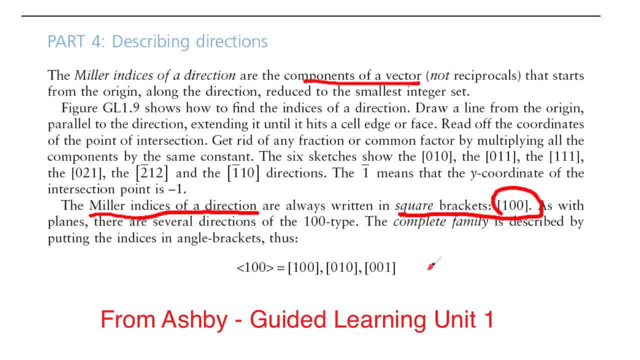 So you'll see them written in two ways: One with the square brackets, as shown here, And then another with these sort of these carrots, these angled brackets, And these are when they're, when it's brackets like this. these are, these are a direction. excuse me, they're a family of directions. And then you can see that this family of directions contains all of these individual directions And, by the way, it also contains the reciprocals of those. 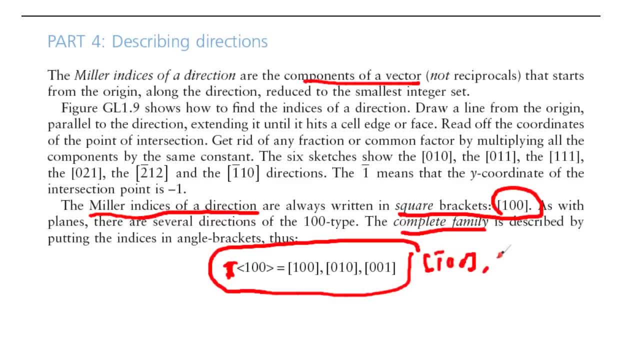 Okay, It contains the one bar, zero, zero. the zero, one zero. excuse me, one bar, zero, And then the the reciprocal of that, the zero, zero, one bar. So it's all permutations of these directions And that's considered a family, that they're all basically rearrangements of these and then also the opposite directions of those. 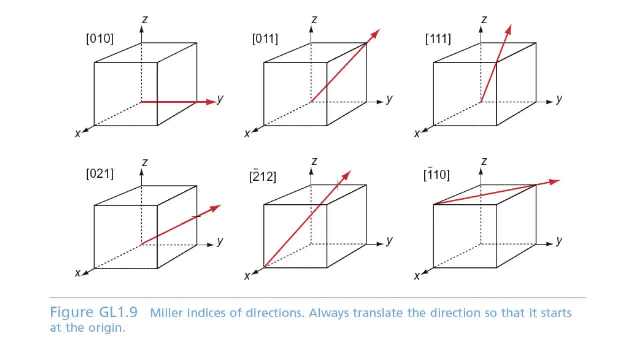 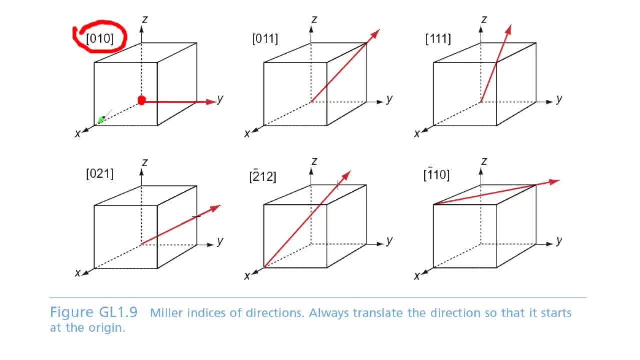 Okay, All right, And then I go 0 in the x direction, 1 in the y direction and 0 in the z direction And I place my next endpoint And then I draw a vector from the origin to the endpoint that I've identified. 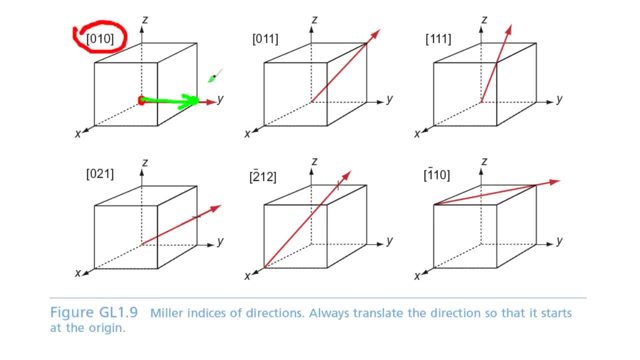 And you can see that that's this red line. Now they extend it beyond the unit cell, which is a little bit confusing in my opinion, as is this one right here, So let's do this one together. So the 0,, 1, 1 vector put the endpoint of the vector at the origin or the originating point. 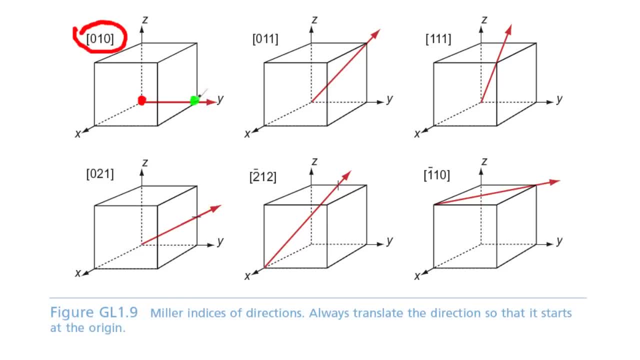 1 in the y direction and 0 in the z direction and I put place my next endpoint and then I draw a vector from the origin to the endpoint that I've identified and you can see that that's this red line. now they extend it beyond the unit cell, which is a little bit confusing in my opinion, as is this: 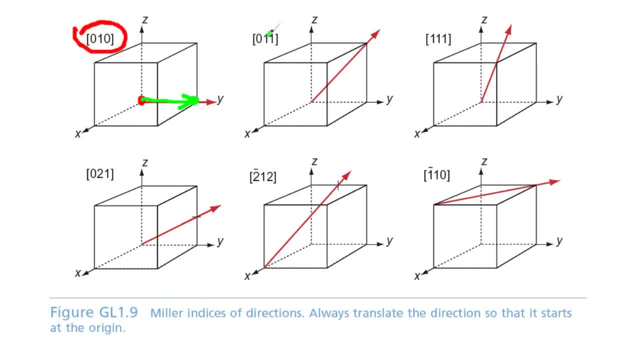 one right here. so let's do this one together. so the 0, 1, 1 vector put the endpoint of the vector at the origin or the originating point, the end of the what is that? the tail of the vector? okay, and then we need to go 0 in the x direction, 1 in the y direction, okay, so 0, I'm starting here, 0 in. 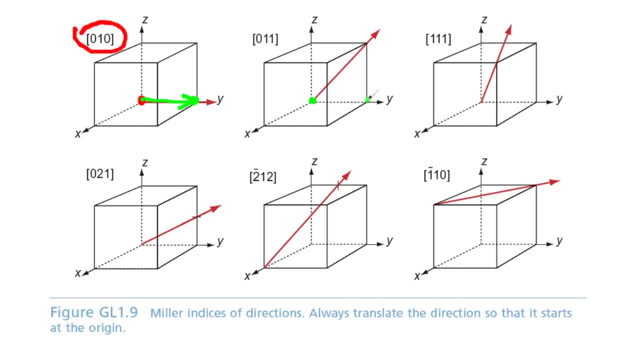 the x direction, I do not move, 1 in the y direction, 1 in the z direction, and then I put the dot there and my vector goes from the origin to this point, right here. now, what's a little tricky is when you're at the origin. you're at the origin, you're at the origin, and then you're at the origin and 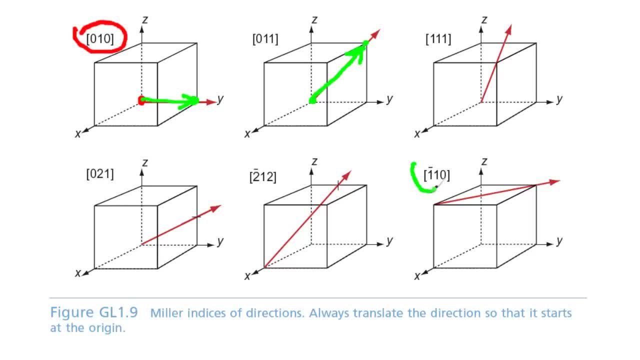 you have in the direction. you have a one bar in the direction or any number barred. so what that means is you basically have to move the origin. if this is a negative number, move it from the 0, 0, 0 point to in that particular direction. so so I'm gonna move this plot, this origin plus 1, so I'm 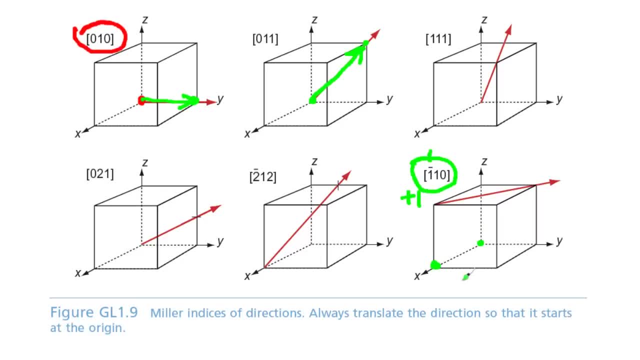 gonna go plus 1, I'm gonna start the vector here. okay, so I can't. I don't think I can erase that other point right here. I don't use a different color. I'll start the vector here and I'll go okay, negative 1 in the x. 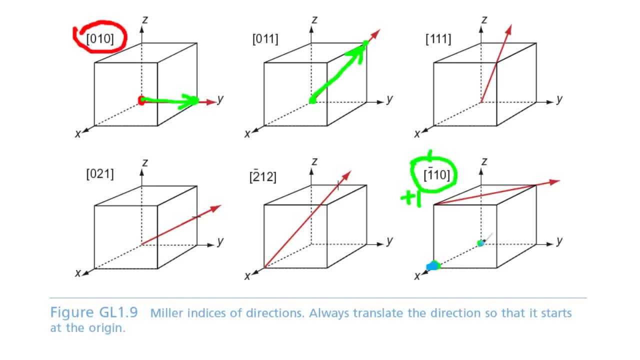 direction: negative 1 in the x direction. oh wait, yeah, negative. 1 in the x direction, 1 in the y direction, 1 in the y direction, 0 in the z direction. and there is my new endpoint. so my direction vector is from here to here. 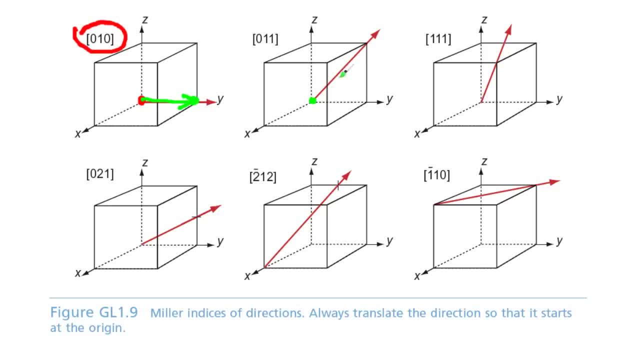 the end of the. what is that? the tail of the vector? Okay, and then we need to go. 0 in the x direction, 1 in the y direction, Okay, so 0, I'm starting here. 0 in the x direction, I do not move. 1 in the y direction. 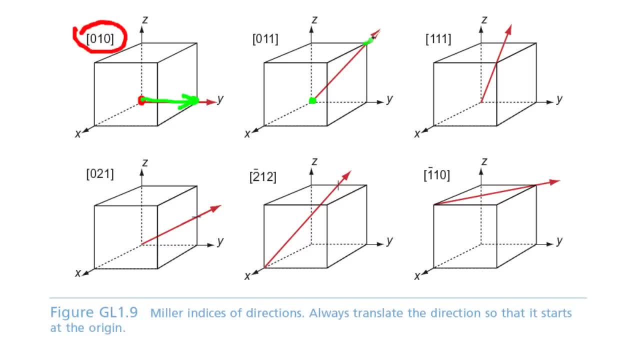 1 in the z direction and then I put the dot there And my vector goes from the origin To this point right here. Now, what's a little tricky is when you have in the direction you have a 1 bar in the direction. 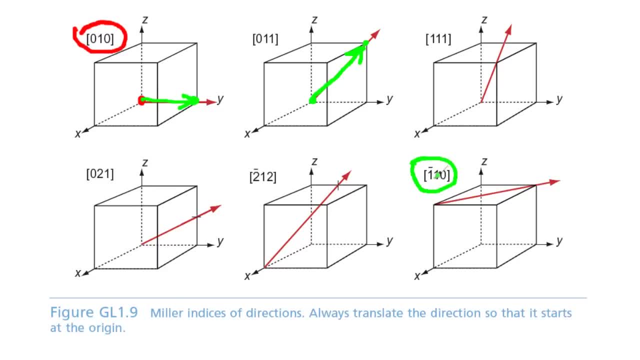 or any number barred. So what that means is you basically have to move the origin. if this is a negative number, move it from the 0, 0, 0 point to in that particular direction. So understand, So I'm going to move this, this origin plus 1, so I'm going to go plus 1, I'm going to start the vector here. 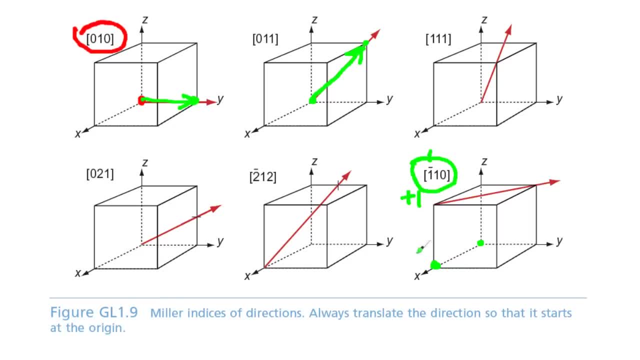 Okay, so I can't. I don't think I can erase that other point right here. I'll use a different color, I'll start the vector here And I'll go: okay, negative 1 in the x direction. negative 1 in the x direction. oh wait, yeah, negative 1 in the x direction. 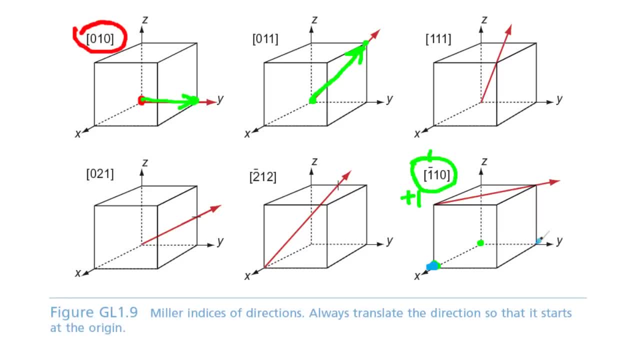 1 in the y direction, 1 in the y direction, 0 in the z direction, and there is my new endpoint. So my direction vector is from here to here. Now notice, they drew that same vector, but they drew it up here. 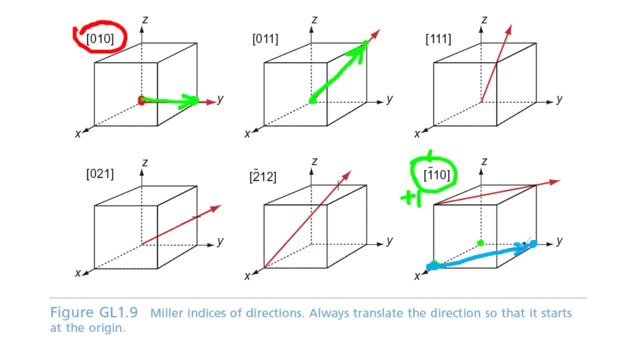 It's equivalent inside this unit cell. It's a little bit arbitrary, but you can see, this direction is the same as this direction. You know. obviously, if we actually drew it out here it would be the same as that. you know, as long as it's parallel. 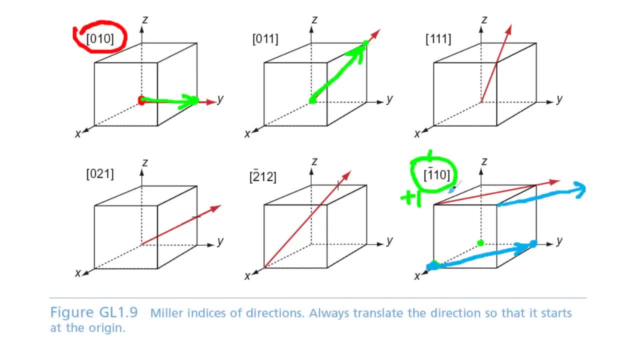 So it depends on where you put the origin. What I would recommend is placing the origin. if there's a negative number, placing it plus 1 in that direction. So here's, let's do this one here. this one's kind of goofy. 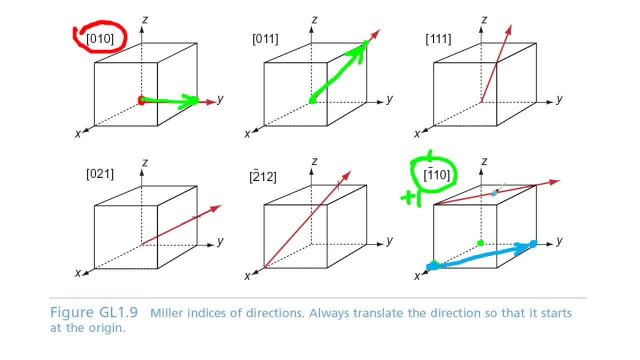 now notice. they drew that same vector but they drew it up here. it's equivalent inside this unit cell. it's a little bit arbitrary, but you can see. this direction is the same as this direction, you know. obvious. if we actually drew it out here it'd be the same as that, you know. as long as it's. 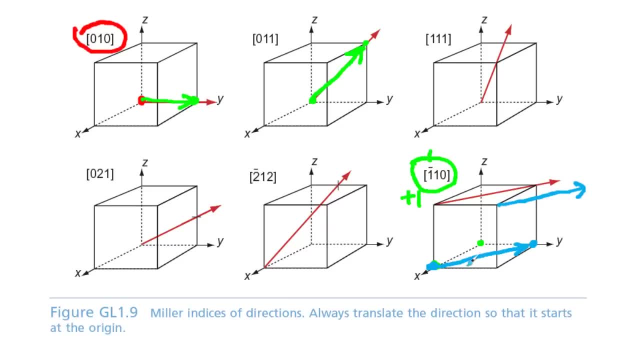 parallel. so it depends on where you put the origin. what I recommend is placing the origin. if there's a negative number, placing it plus 1 in that direction. so here's, let's do this one here. this one's kind of goofy. now, when you have greater than 1 inside here, what I would recommend doing is pulling that number out. 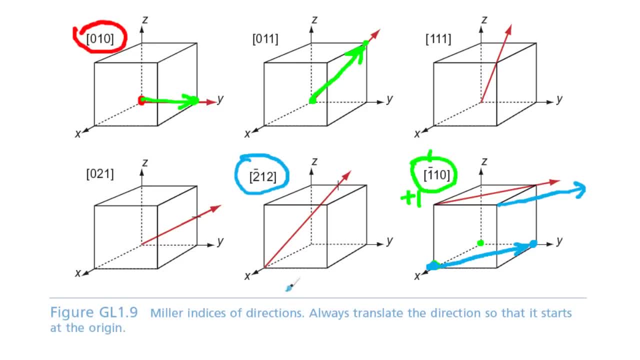 so that you know, common factor out and I would say 2, pull the 2 out 2 and do 1 bar 1, half 1 to get that same direction. so you're saying 2, 2 times this direction. that's 2 is just the magnitude of. 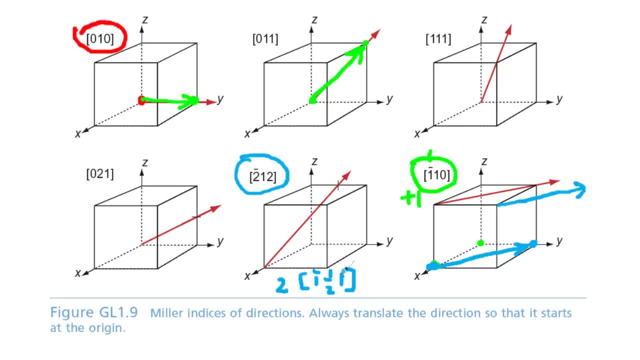 the vector. so what I would recommend to do is to say 6 or 7. this would be half the size and direction of the vector, but the direction would be the same. okay, so we need to go, since we have one of one bar in this x place right here, the x, y, z, I would personally 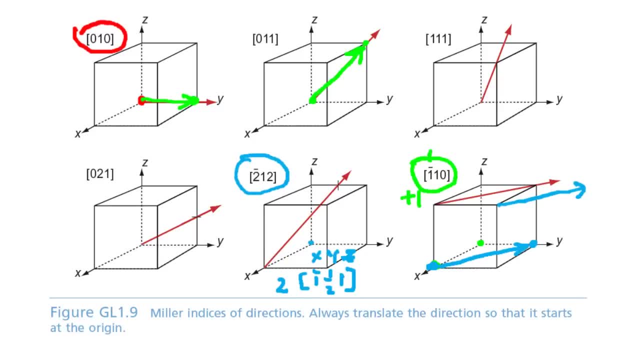 add 1, so I would start at 0, 0, 0, I would add 1. so now here's my new origin. I use a different color, I'll use green. here is my new origin and I'll start from there. so I'll go negative 1 in the x direction. 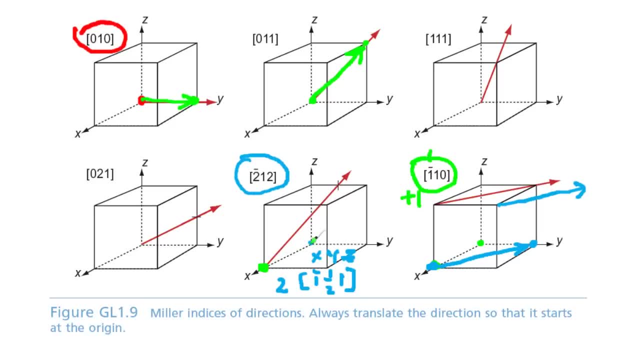 negative. 1 in the x direction. I'll do one half in the y direction. one half, that will put me right here. then I go one in the z direction. that will put me right here. so the direction vector would be from here to here. see, they draw the head outside there and that's that makes it confusing, in my opinion. 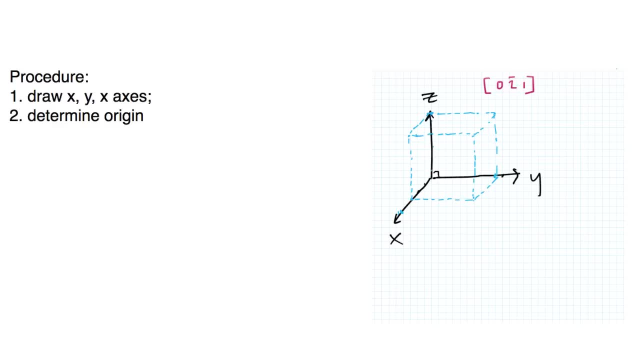 anyway, I hope this helps. okay, let's go over the procedure here. so let's say the first thing that you want to do is draw the xyz axes. the second thing is to determine the origin as the, the tail of your vector, the direction vector, okay, and in this case, if there is a negative, 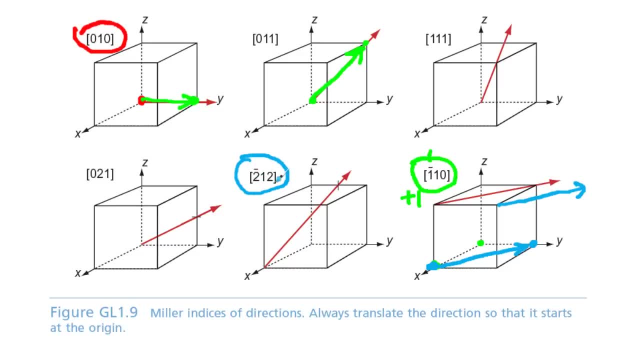 Now, when you have greater than 1 inside here, what I would recommend doing is pulling that number out so that you know common factor out and I would say 2, pull the 2 out and do 1 bar 1 half 1, to get that same direction. 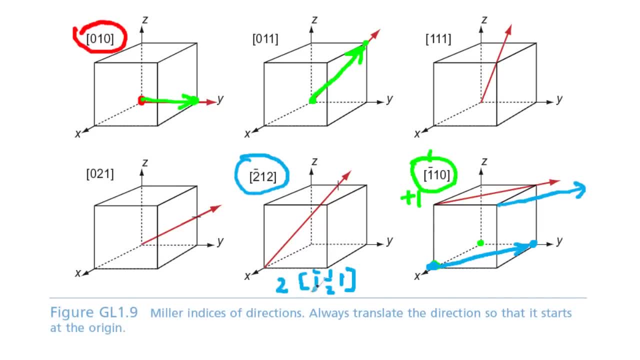 So you're saying 2,, 2 times this direction. 2 is just the magnitude of the vector, So this would be half the size of the vector, but the direction would be the same. Okay, so we need to go, since we have 1 bar in this x place right here, the x, y, z. 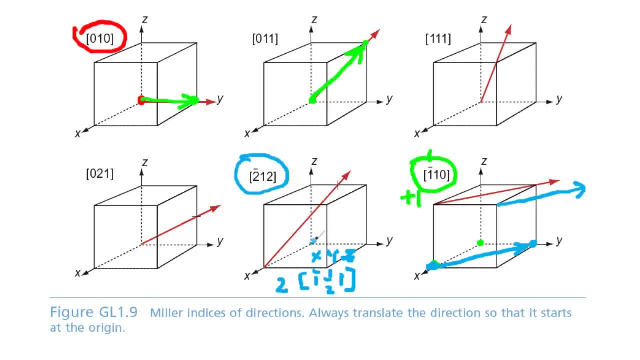 I would, personally. I would add 1.. So I would start at 0, 0, 0.. I would add 1.. So now, here's my new origin. I'll use a different color. I'll use green. 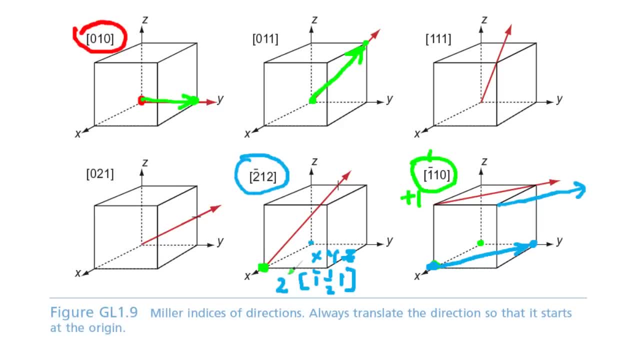 Here's my new origin And I'll start from there. So I'll go: negative 1 in the x direction. Negative 1 in the x direction. I'll do 1 half in the y direction, 1 half. That will put me right here. 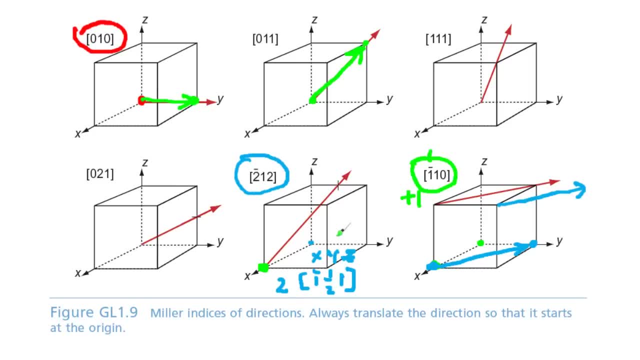 Then I go 1 in the z direction. That will put me right here. So the direction vector would be from here to here. See, they've drawn the head outside there and that makes it confusing in my opinion. Anyway, I hope this helps. 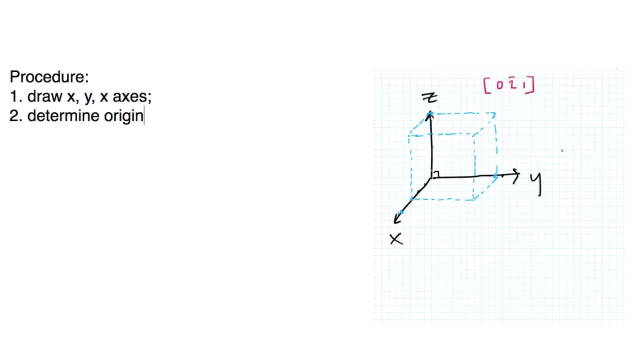 Okay, let's go over the procedure here. So let's say the first thing that you want to do is draw the x, y, z axes. The second thing is to determine the origin as the tail of your vector, the direction vector. 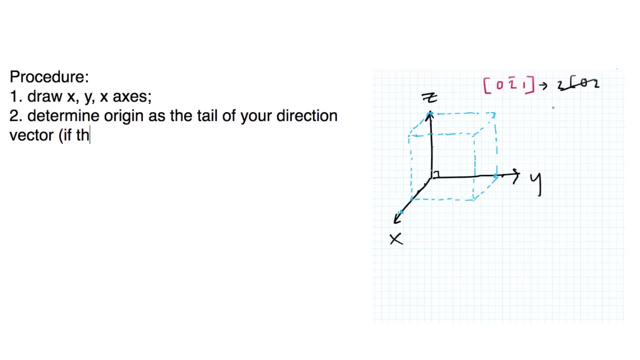 Okay, and in this case, if there is a negative number in the direction vector, move the origin in the positive direction for that axis, And then the next thing you want to do is determine the endpoint, And you want to do this.